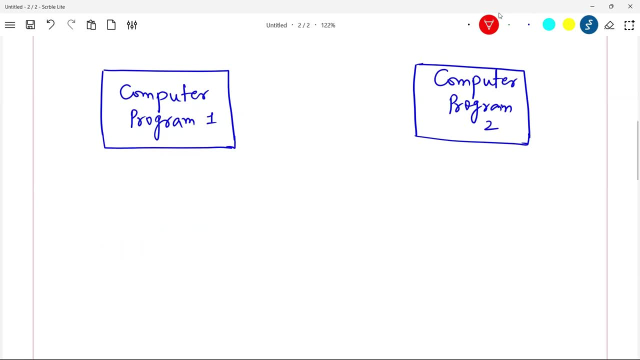 Suppose this is a computer program on the left hand side. On the right hand side is another computer program. This is program one And this is program two. Okay, The name of the program one is, let's say, Amman dot py. Okay, Amman dot py. In Amman dot py, I want to add two numbers. 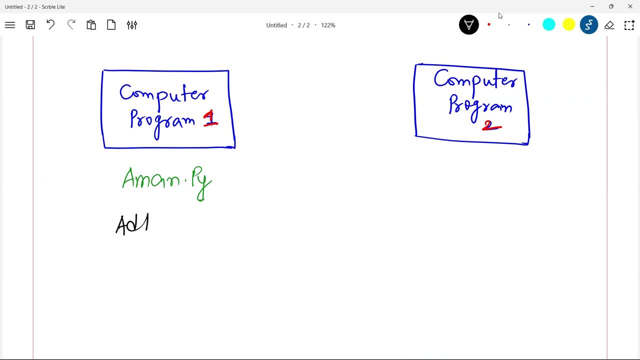 What I want to do. I want to add two numbers. Okay, add two numbers. It's a very simple task I want to do in my program, But for some reason I don't want to use Python, some function, or I don't want to write the logic. I'm lazy to do that. Okay, So there is a. 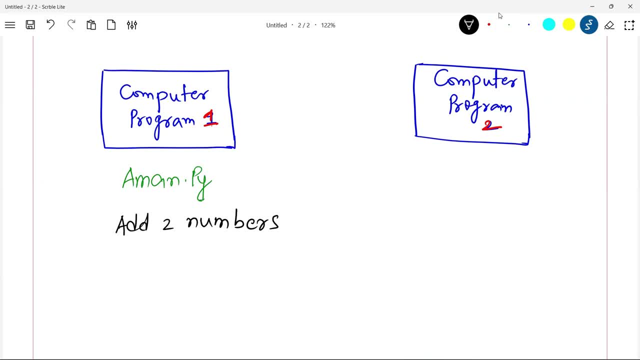 provision through which I can ask this computer program to. So what I can do, I can ask this computer program to: Hey, can you add two numbers for me? And the program will say me: okay, give me those two numbers. At the moment I give those two numbers, this second program will say me: okay, give. 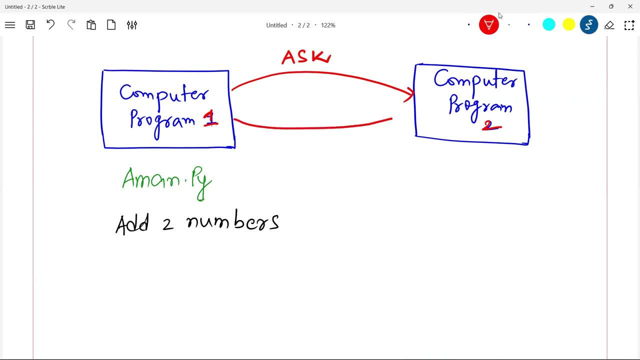 me those two numbers. At the moment I give those two numbers, this second program will say me: okay, give me those two numbers. At the moment I give those two numbers, this second program will return me the response, which means two numbers added. it will give me as output: Okay, So what? 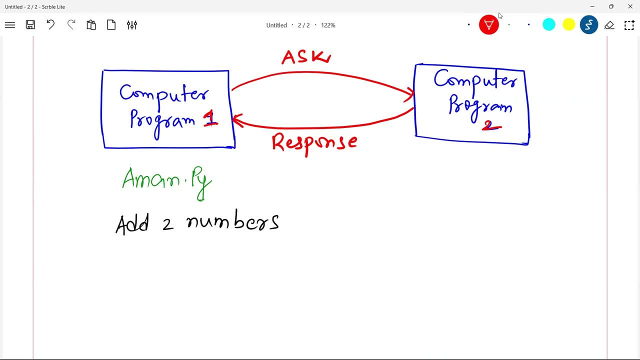 has just happened is I'm using the logic written in program two in program one. Okay, And this entire concept is known as concept of API's. In this case, this is your root program, main program And right hand side program. you can think of it as an API. So what is an API? an API is a place. 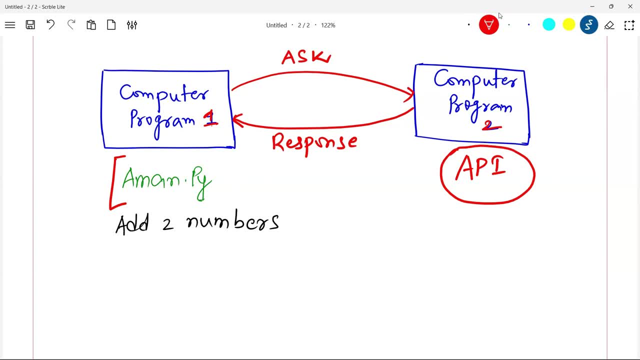 or is a program that you use in your program if you are lazy to write code or if you don't want to write code that has been written by somebody else. So you ask question in a particular format and you get response in a particular format. Now, here I am saying, adding two numbers. 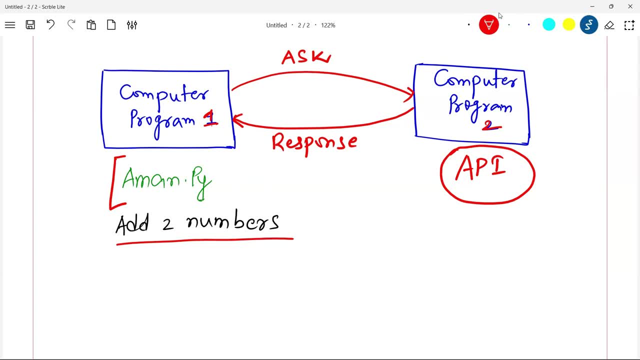 so you cannot ask add three numbers, or you cannot ask multiply two numbers. you just have to ask: Hey, give me the addition of these two numbers. So format is fixed, what you can ask and what you can get in return. that format is fixed. Okay, let me show you one simple example. 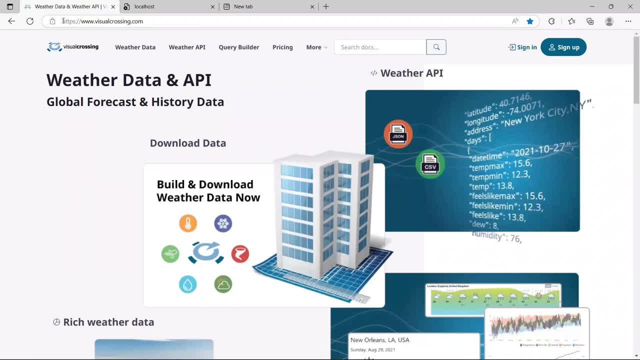 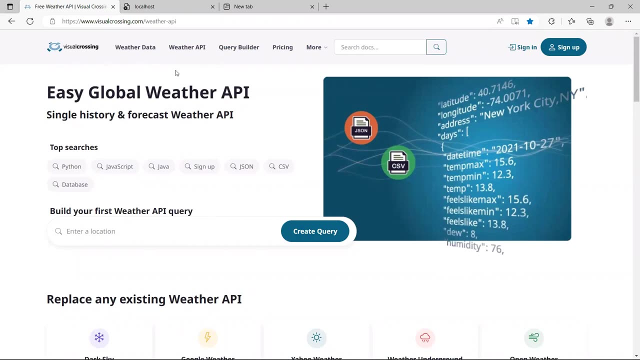 of how an API looks like. So come here. I am in a website, visualcrossingcom. Okay, let me enter one more time Here. I will click this link, whether API, so I'm clicking this weather API. So this particular page is called endpoint of an API. So what is an endpoint of an API? 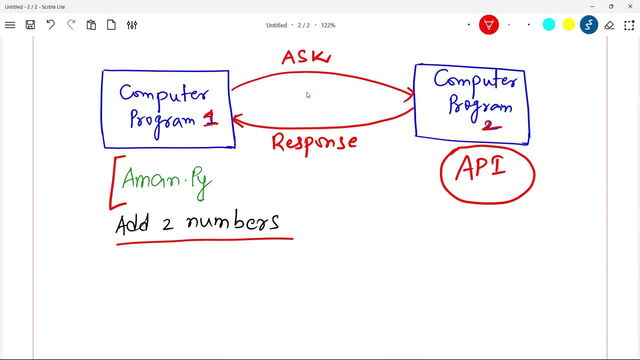 For asking your question, you have to go to the Endpoint of an API. So what is an endpoint of an API? For asking your question, you have to go to the Endpoint of an API, A point where API receives questions. Okay, so in this case, API is receiving: 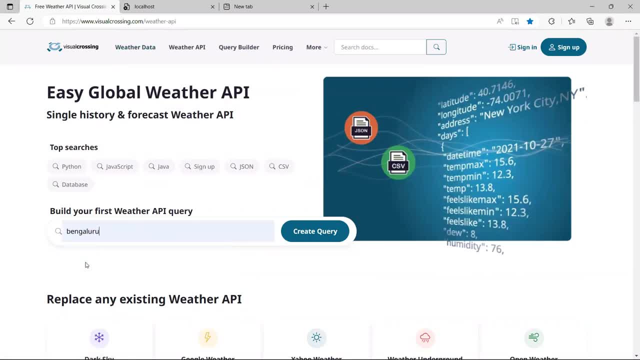 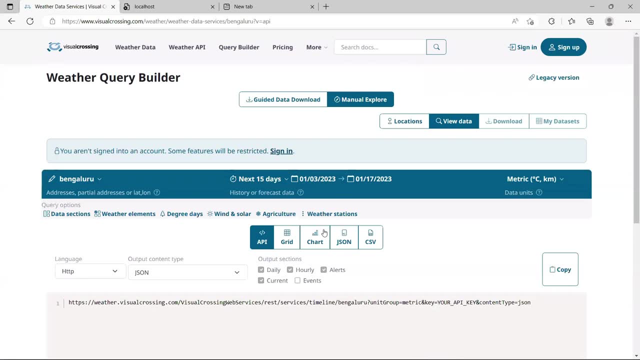 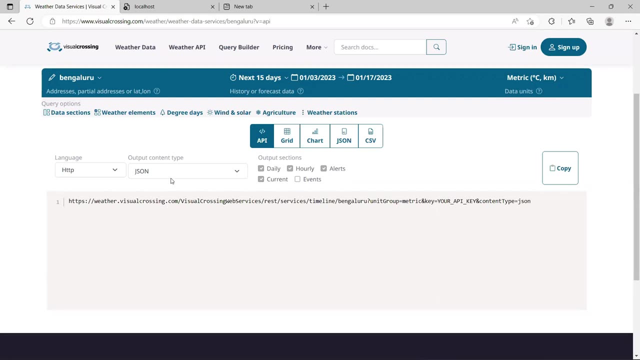 question here. So here I will enter Bengaluru, So Bengaluru is the city for which I want to know the weather updates And I will say create query. At the moment I say create query, the query has gone to the API and response also I receive within minutes, within seconds. So here you can say I can. 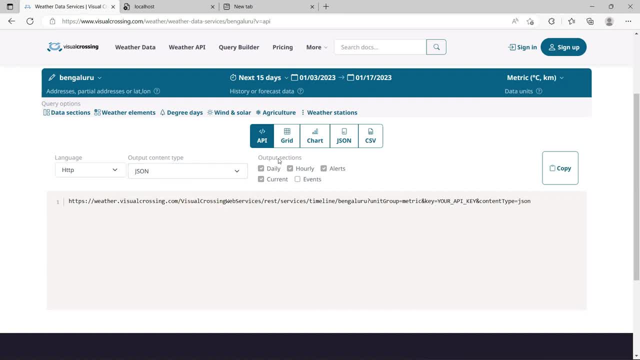 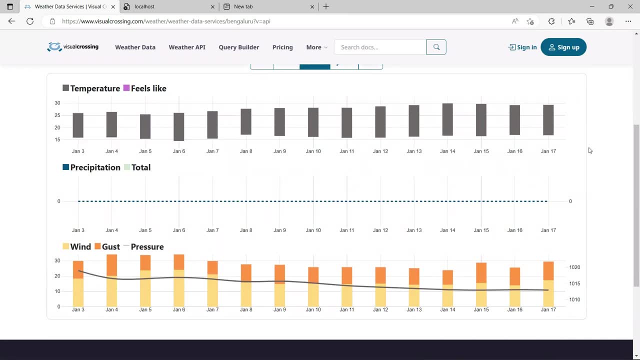 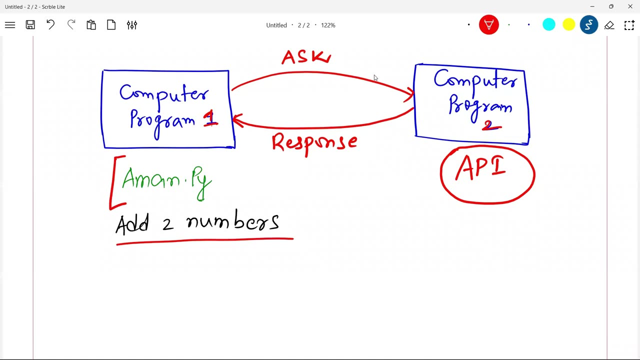 get the response in JSON, CSV, Excel, etc. And if I click on this chart, right, so I have data of Bangalore. So what is the temperature, What may be the forecast, etc. Okay, all these things I have. So what has happened? just now, I went to the API endpoint. 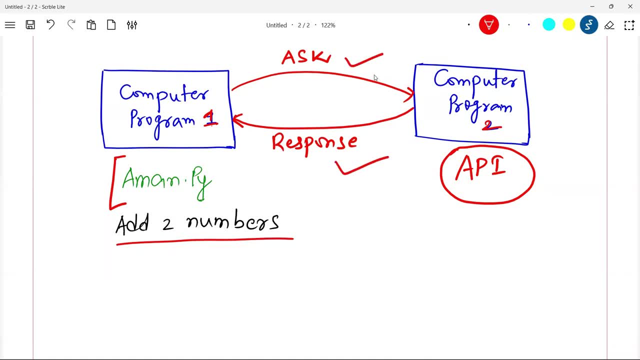 I asked my question and I got my response, But remember, there is a format fixed. I cannot ask any random question or I cannot give any random input. Okay, what is an API endpoint? API endpoint is a place where you go and ask your question. Okay Now. 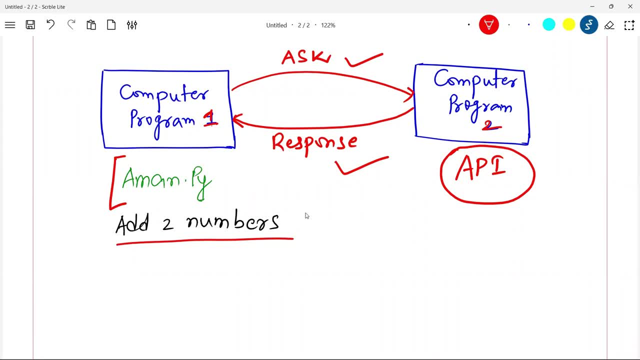 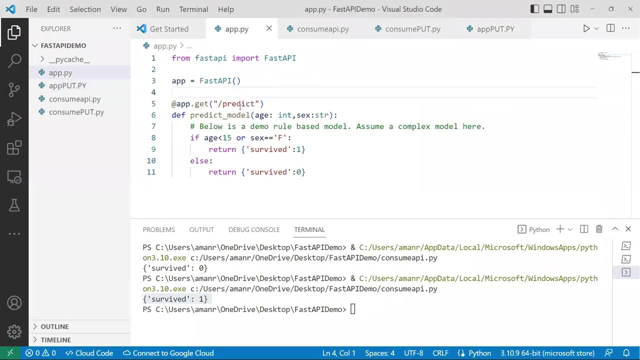 let's try to understand how we can build our own API in Python in few lines of code, just few lines of code. Okay, So I'm going to my Visual Studio guys and I'm having a file here: apppy. Fine, I'm installing a package- fast API. you can install this package as well. very simple. 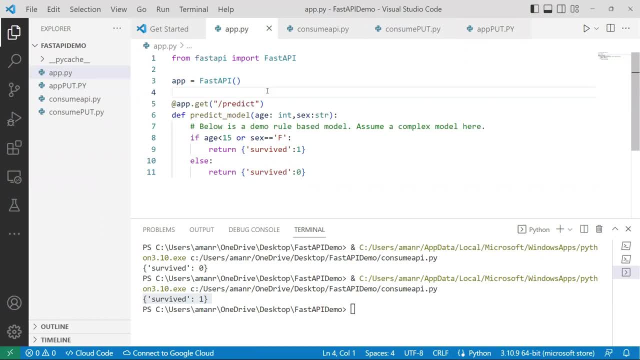 to install And I'm assuming my machine learning model is a very, very simple model. So line number eight to 11.. What I'm, what I'm highlighting now, is my machine learning model. So what my machine learning model does. it takes two parameters: age of the person and sex of the person. 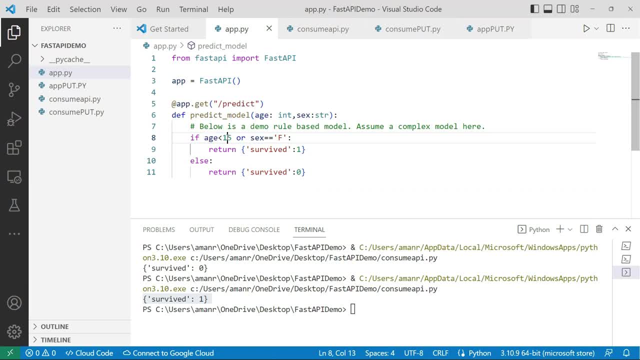 and it is its suppose that any data set. So based on the age and sex, it will say whether the person survived or did not survive. Okay, so this is just simple rule based machine learning model. I'm saying below is a demo, rule based model. as you make complex model here, fine, 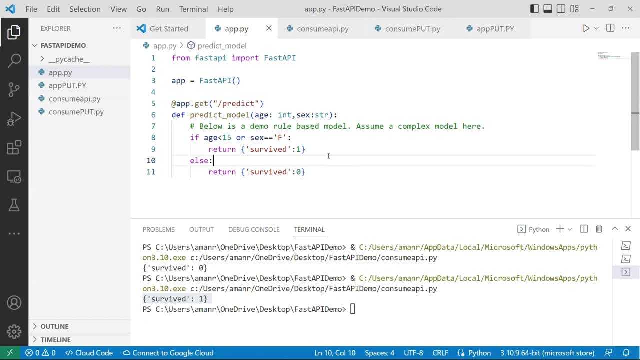 But I will host this in the API for Okay, so what? what I'm trying to do is I will try to give a age and I will try to give a sex and try to find information based on whatever logic I have written here through this API. so for: 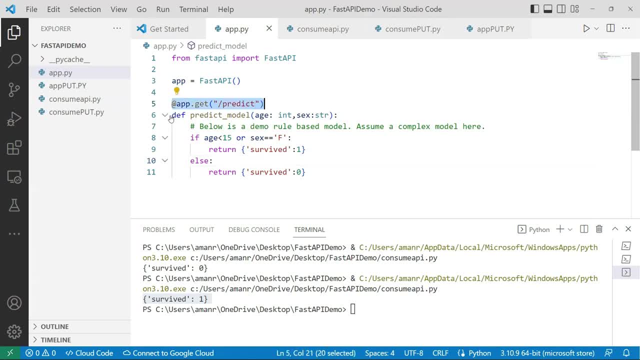 that there is a decorator, I have written slash, predict, then definition of the of the function that runs inside predict. so very simple logic here. just you have to initialize fast api, create a decorator and write your logic. okay, so this is my code. in my desktop there is. 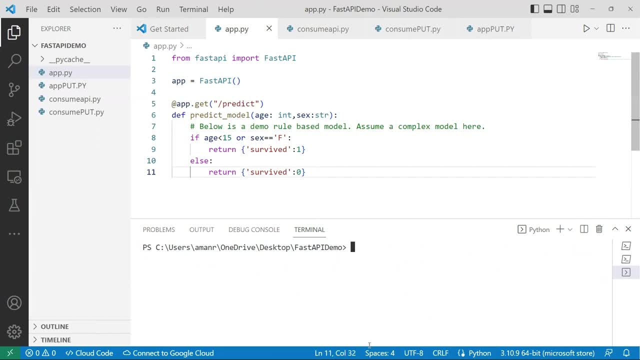 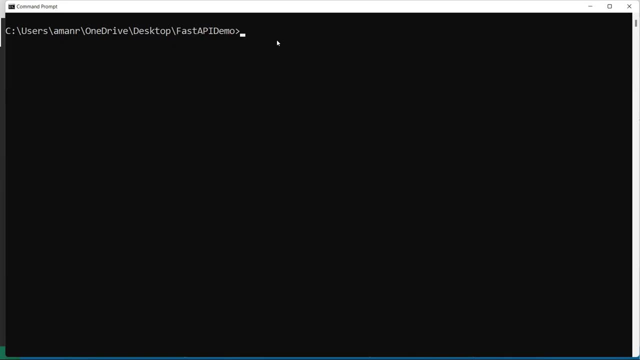 a file called fast api folder is there and this file is there. okay, and let me go to my command prompt and I'm inside desktop and fast api folder, okay, in Windows machine. I will just go here and say: python 3m uvcon. uvcon is the server on which it will run app. 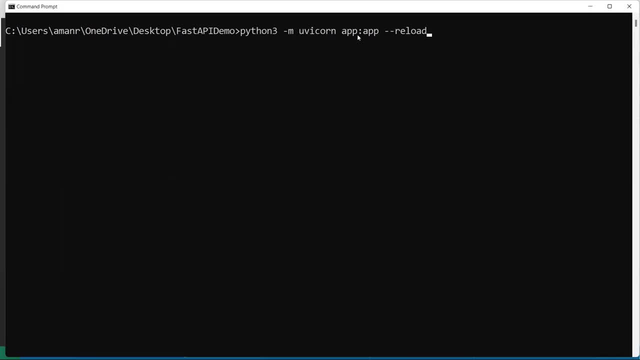 app is the name of your file here, apppy is the name, colon app. and then reload. okay, you can run this command as well. you say enter at the moment. you say enter, it will say say you uvcon running on 127.0.0.1 8000. that is your local host. 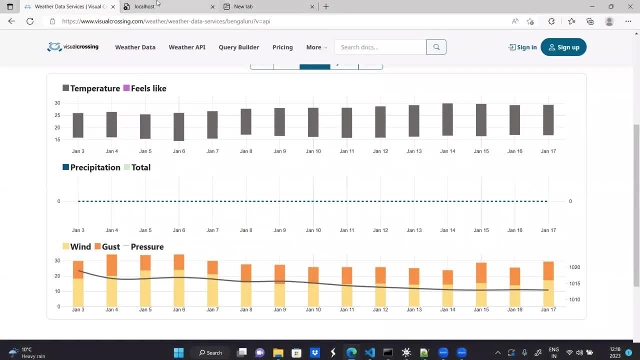 let's go to my command prompt and I'm inside desktop and fast api folder. okay, in windows machine I will just go here and say: python 3m, uvcon. uvcon is the server on which it will let me go to my browser and try to open that, that address. so localhost, 8000, 8000. so if 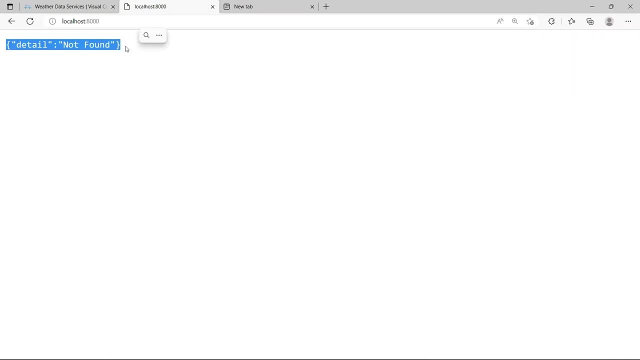 I do like this. you will see details not found why? because we are not asking any question. api is running here, but we are not asking any question. okay, so just to showcase you, just to demonstrate you, it is not not how we do in the real world, but we do in the development. 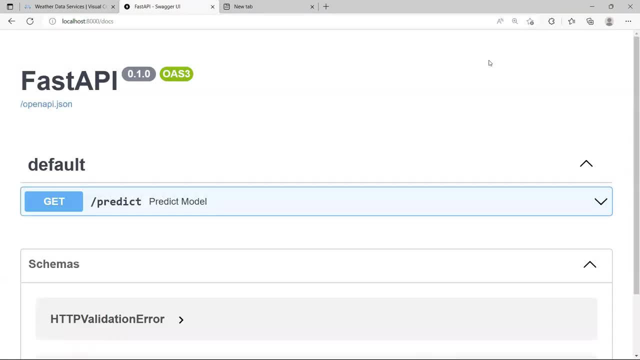 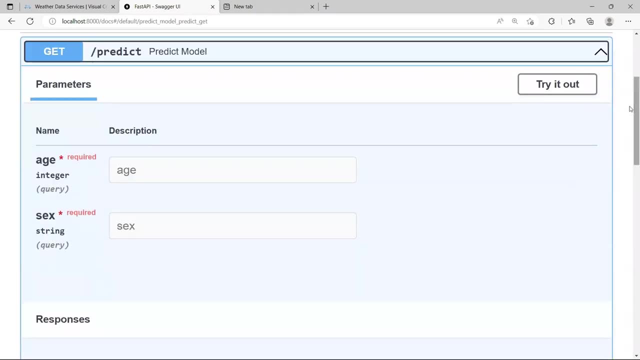 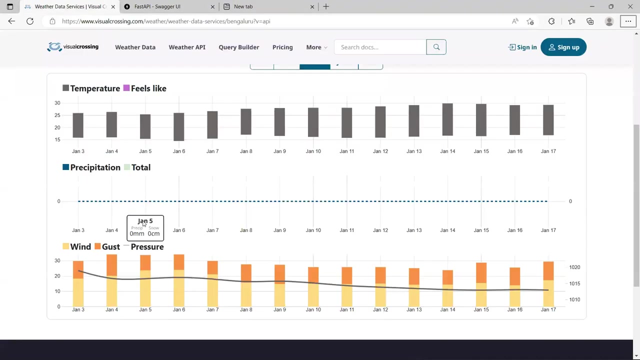 process. okay, so if you go to the docs right, then you will see a UI like this. fine, in this image, maybe, if you click on this, get right and you click on this, try it out. so here you can enter your age, for example 21, and I will say f, so it will run based on our FL logic. 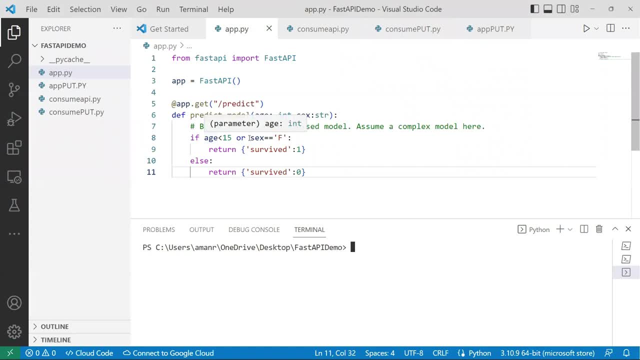 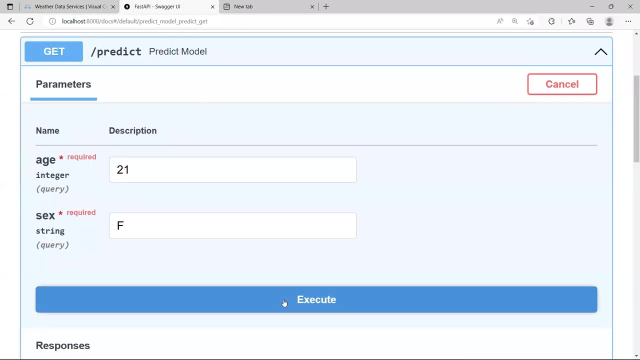 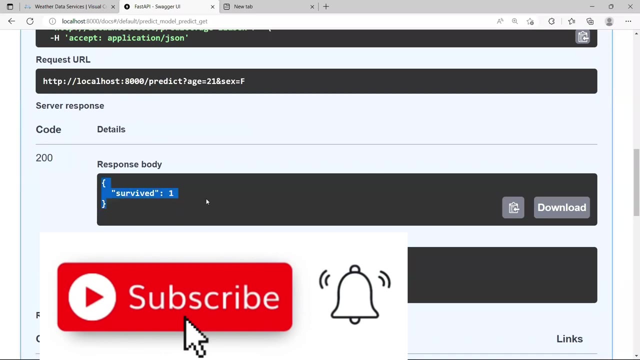 whatever we have right written here, so any anywhere where sex is f, it will be a survived case. okay. so let me go to my gear and execute it so I should get a response. you can see here response: body survived is one. okay, so that is what we expect. so this api is working. 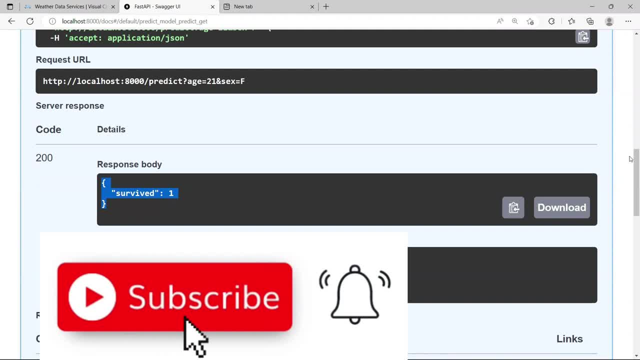 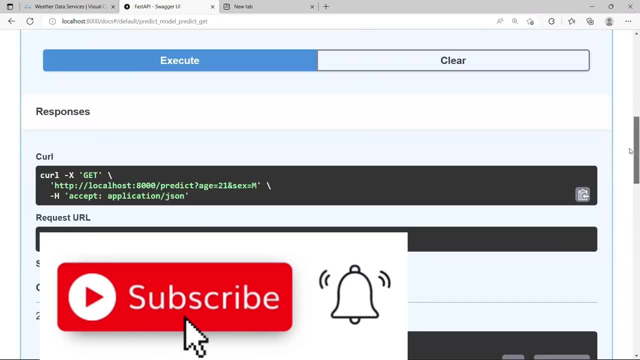 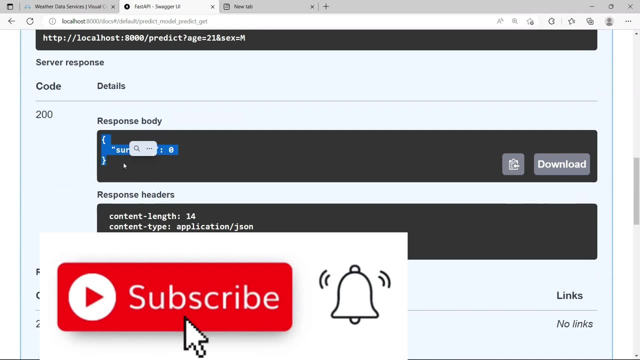 fine, and, as you can see here, if i go ahead and make the this as mail, then it will be survived zero, because that is the logic we have written in f, else loop. okay, so this is how you develop an api using fast api, but there are things to learn here, so, as you can, 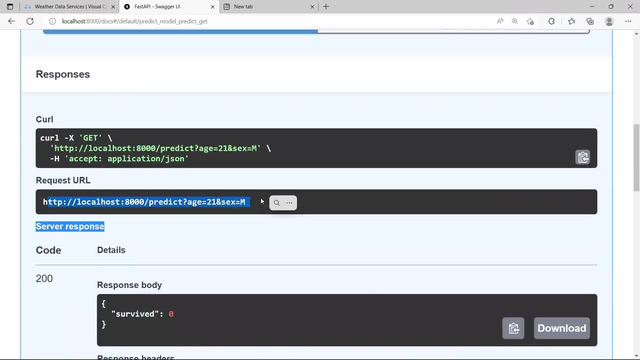 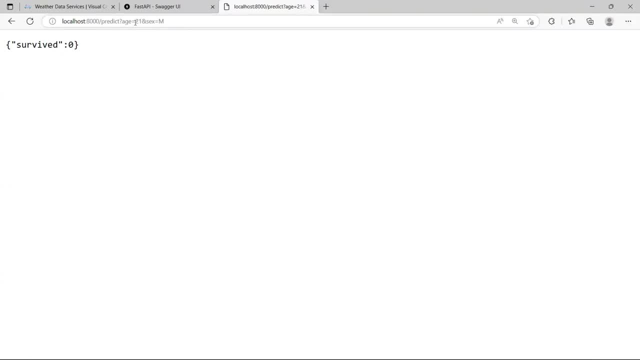 see here guys, request url goes like this: so this is my request url in the url. your age and sex are going as input in the url. your age, whatever age you give, whatever sex you give, that goes in your input. and then you get survive. for example, if i make this as: 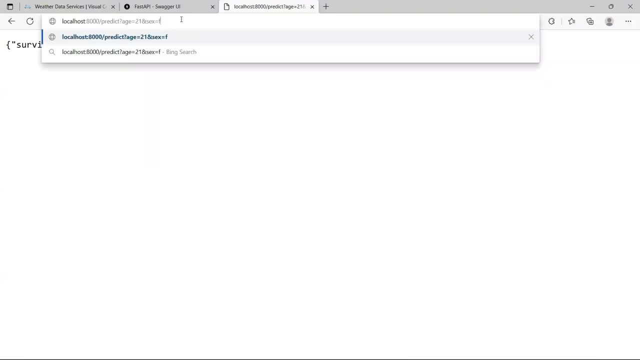 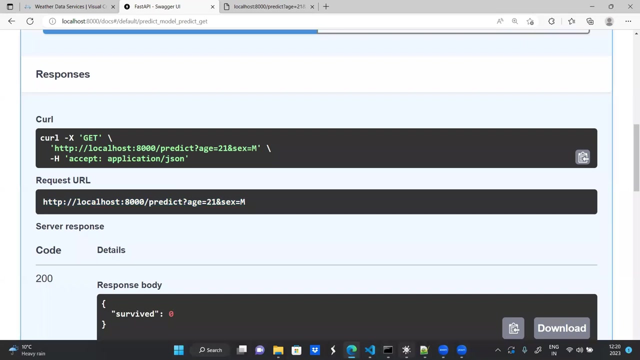 f, it will say me: capital f, actually let me make it f. then it will say me: survived one because female is surviving based on our reference logic. but whatever we did now, that is for development purpose, testing purpose, if our api is working fine. suppose i give you the example of two python programs, right? suppose i want to call that api in a python. 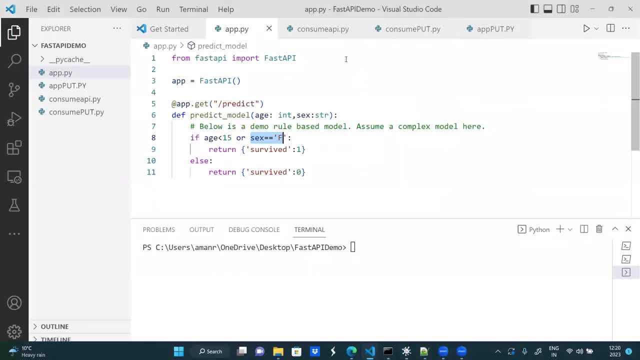 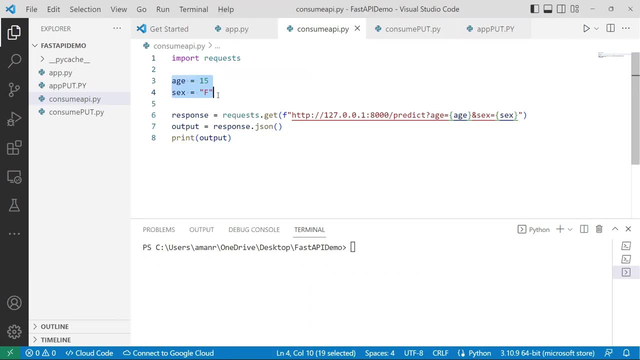 program, then how can i do that? let me show you that as well. consume apipy is another file i have here. here i am importing requests. then i am saying: my age is this, sex is this? go ahead and call this url. so, as you can see, this url is very similar to the url i showed. 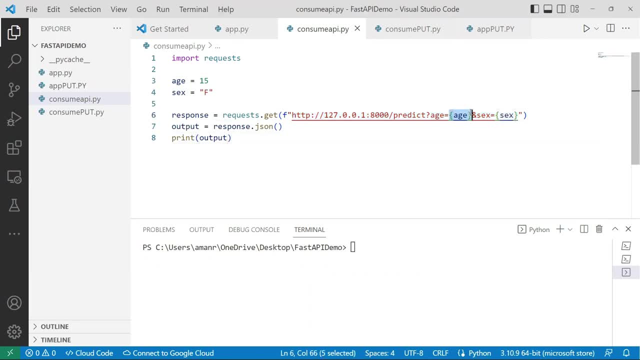 you now in the browser, just that we are passing agent sex as the variables here. okay, at the moment i run this, you will see that i will get a response: survived one or zero, based on whatever the logic. okay, so here, survived one is the response, fine. so whatever way we are doing this particular development, guys, 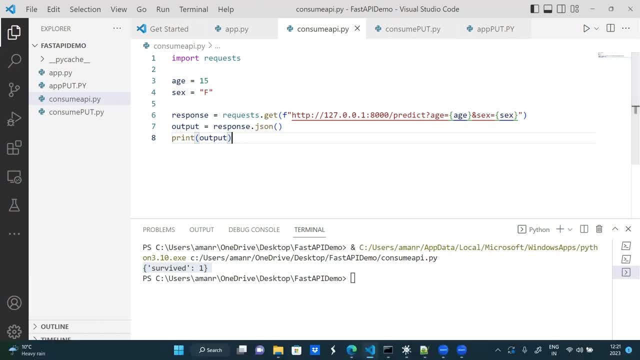 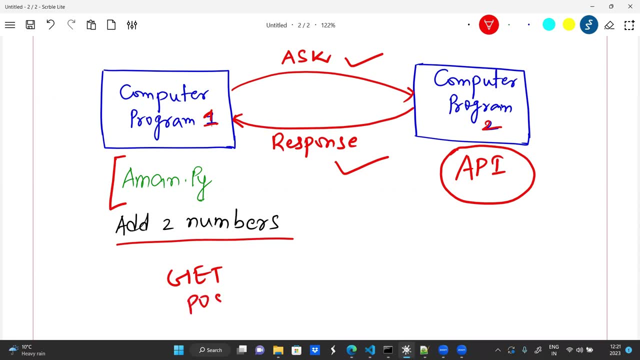 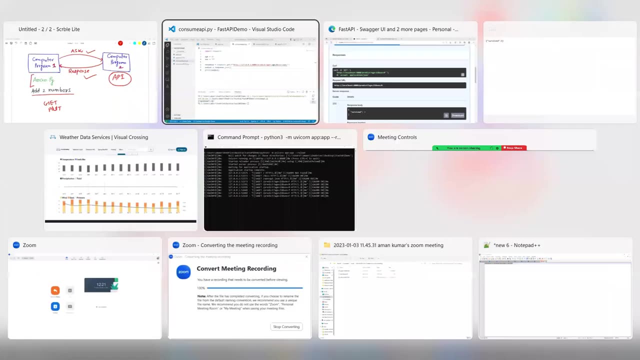 this is known as the gateway. okay, so there are two ways in which you can. you can build your api or call your api. one way is called gateway, other way is called post way, in the sorry, put way, put way, not post way put way. okay, and here what you can see is we are passing the 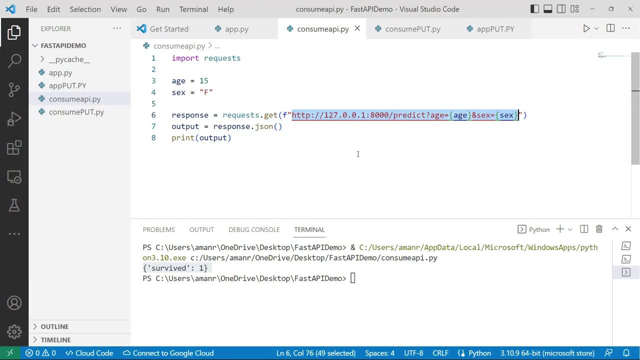 url in url, we are passing the variable, but this is not a very good practice. okay, so there is an another way in which we can do that, and that is by not passing in the url the data. so, for example, we can write a code like this: there is a package called pedantic i am using here, but there are. 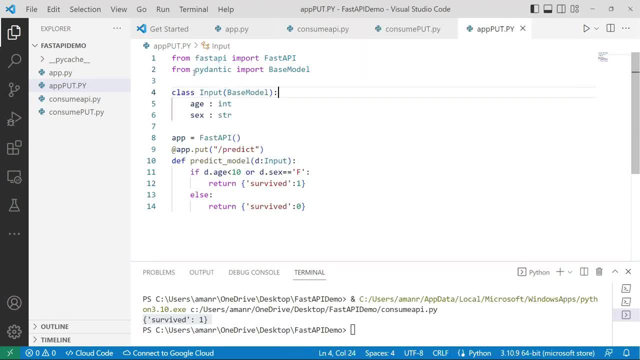 other ways of doing it. okay, so from pedantic pidentic you call it pidentic. okay, from pidentic, you got a base model. in this base model, you can give your inputs and same way you can write your logic. the difference between this method and previous method is just the way you are passing. 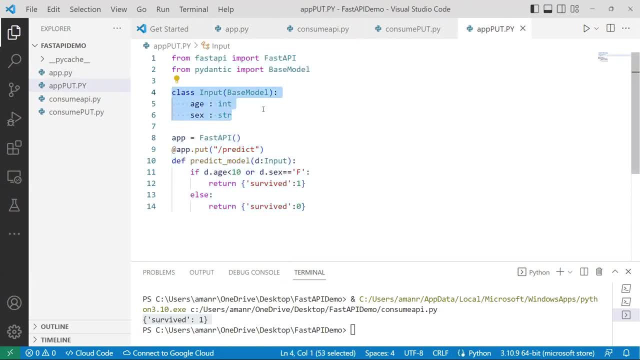 your input to the api. okay, so this is supposed to be more protected? why? because if i want to consume this api, then i will create a payload like this. okay, so you are saying consume, put, you are seeing this payload and i will pass. data is equal to payload. in this way, my api will be protected and my data. 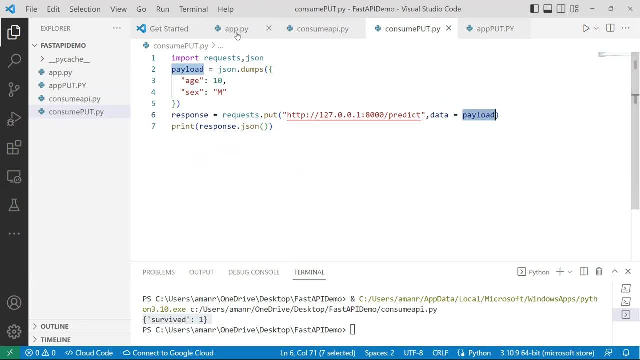 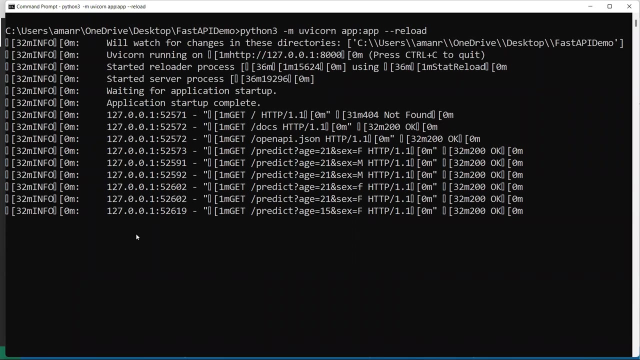 will not be passed in the url, like it is getting passed in the previous method. okay, so few important things to remember in the concept of apis. for using an api, it should always be running. for example, this api is running here. suppose i stop it. i press ctrl c so api is stopped. now i can't. 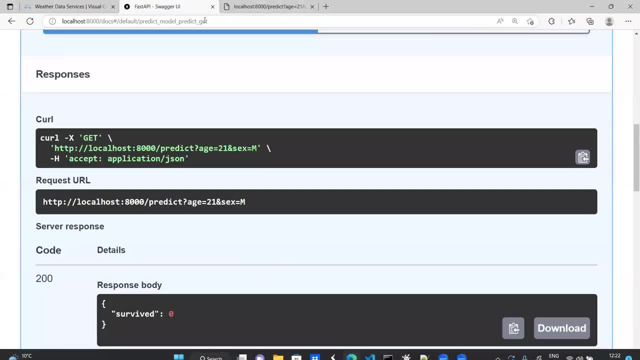 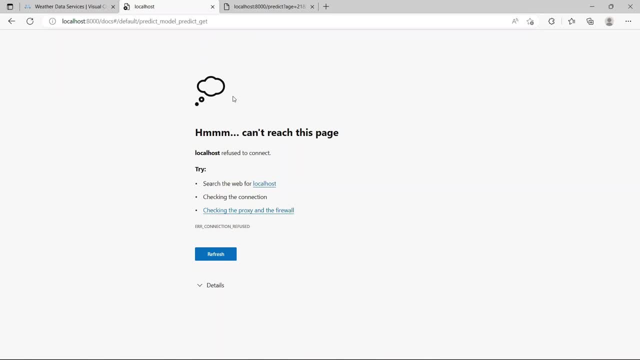 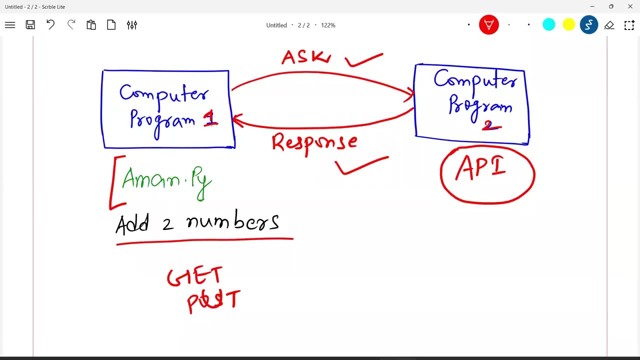 go and ask any question to that api because that service is stopped. okay, so if i, if i click this right, then it will say it cannot reach that because i have stopped that. so to to you know, ask any question to the next program. your api should be running and there are two main ways of doing that. i showed you you should not pass. 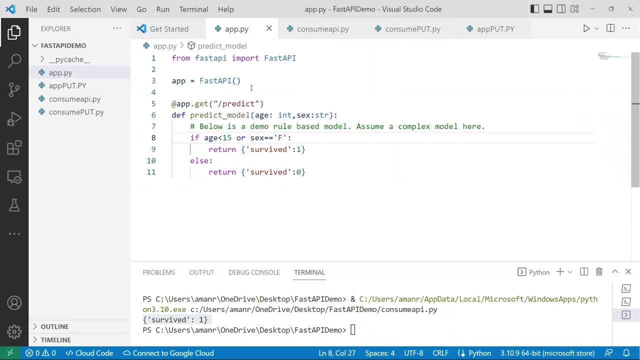 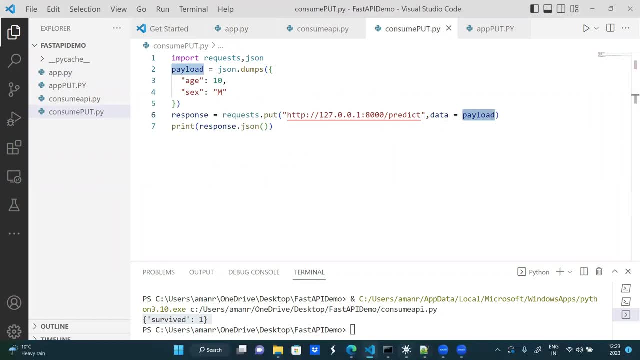 your queries or parameters in the url. that is not safe, so you will want to use the second way, and in practical, more sophisticated ways as well. okay, so what all we learned? let's revise it quickly, guys, and i will see you in the next video. bye, bye, bye, bye, bye, bye. 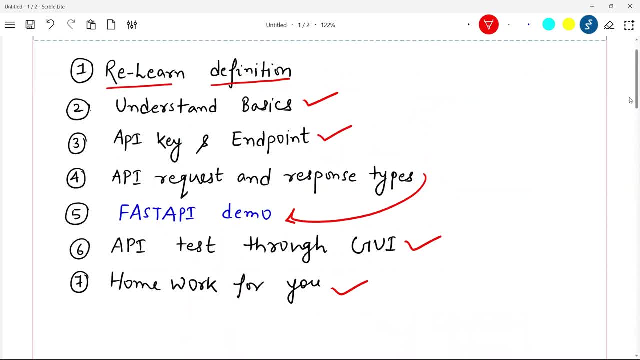 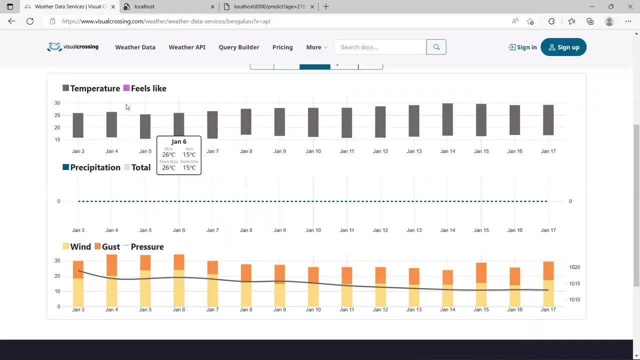 will give you a simple homework. we learned the definition, we understood basics, keys and endpoints. okay, keys, i did not tell you. key is basically a way to protect unwanted requests. suppose i went to this weather data and i gave bangalore and i got the output right. so somebody can misuse it. somebody can do it multiple times or misuse it or sometimes. 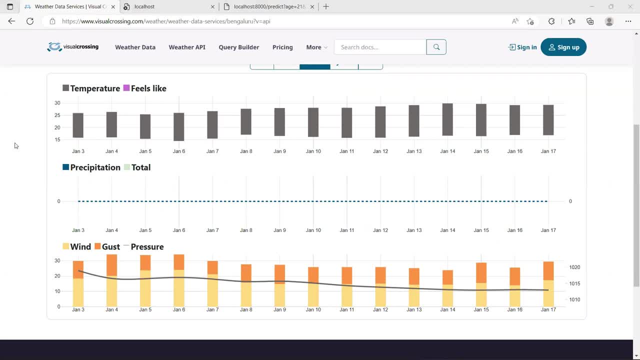 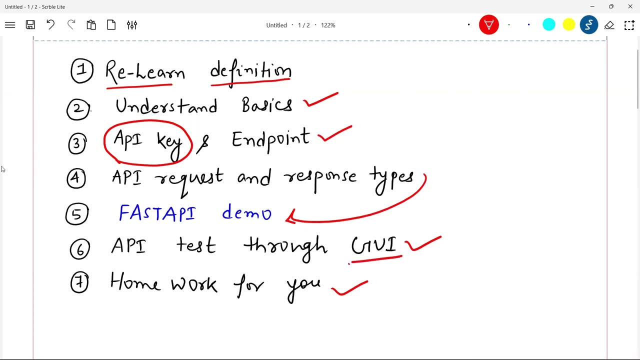 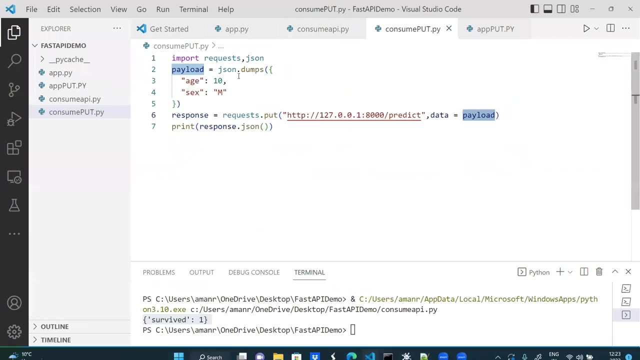 some people want to charge their apis with some money for those purposes. you know, key concept is their api key. okay, request and response type. i explained you demo and then we learn how to do using gui homework for you guys. i built a simple model here. if else model, please go ahead and try to host a machine learning model.